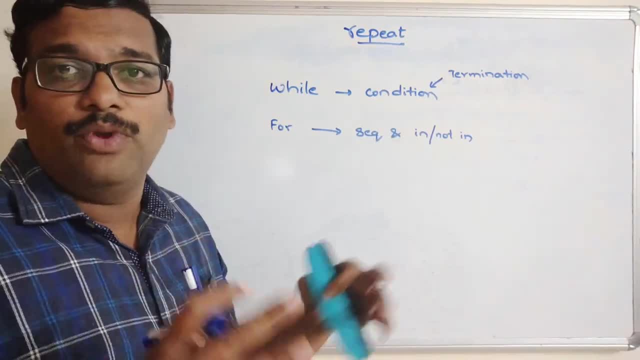 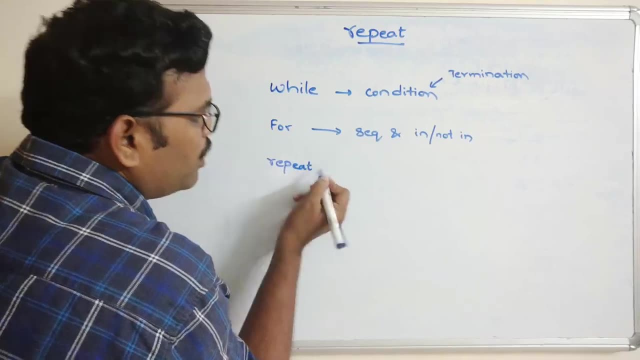 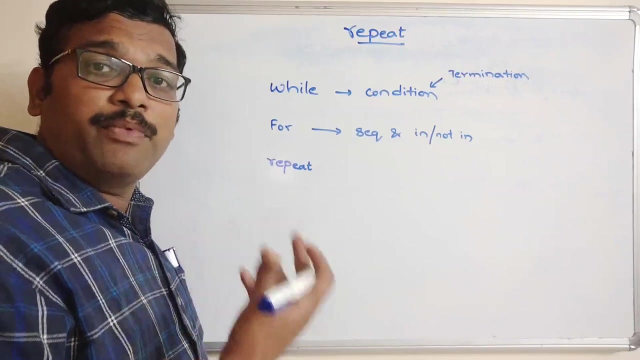 immediately the termination will be. I mean, the iterations will be terminated. so this is for fun. look now what is a repeat. so we are saying that repeat is also a category of iterative statements. that means here also the same set of instructions will be keep on executing multiple times. so here, what about the? 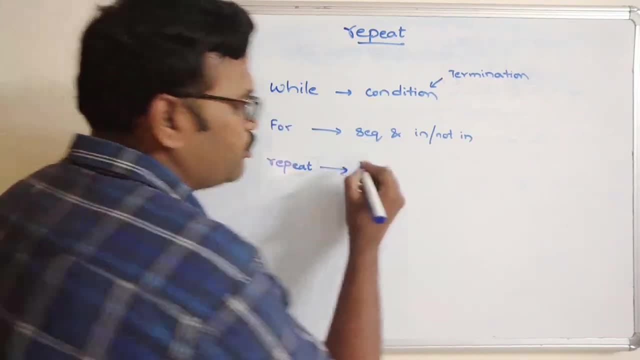 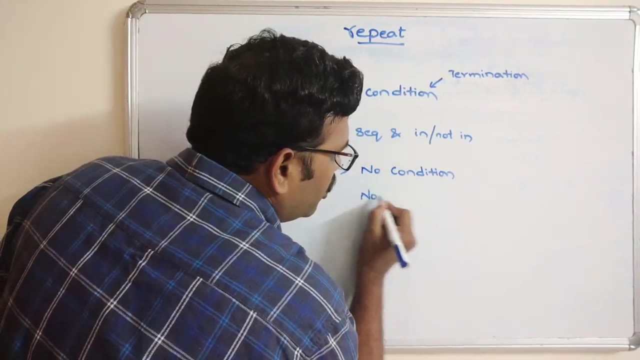 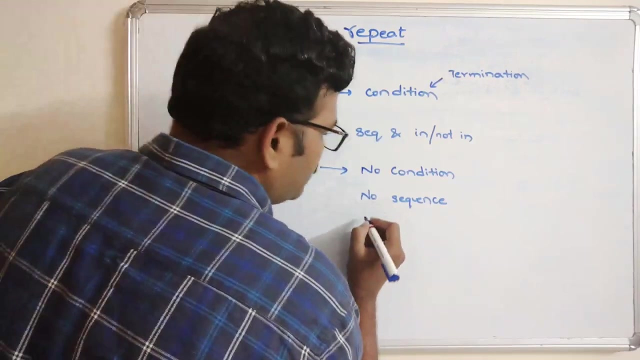 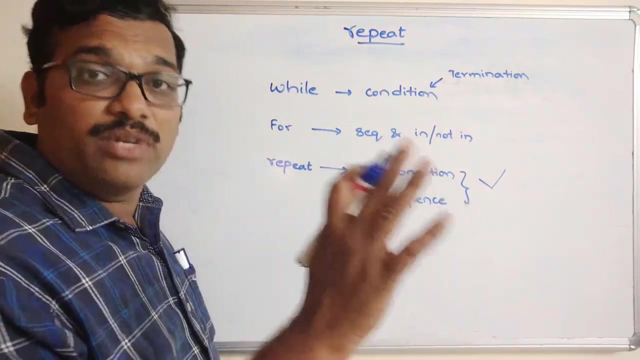 termination. so when the there will be termination? so here there will be no condition. so we are not able to write any condition and also no sequence. so we are also not going with any other sequence. so just so this is not possible, right? so we are not writing any condition and not any sequence. so when 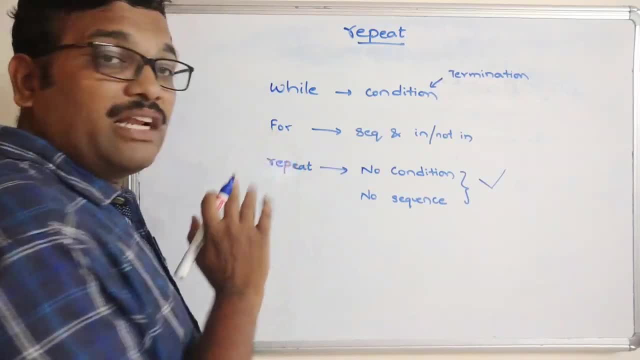 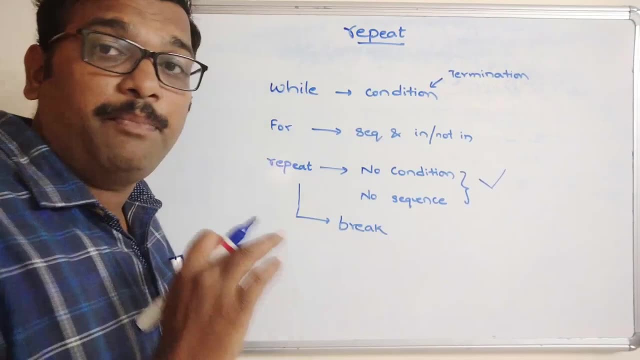 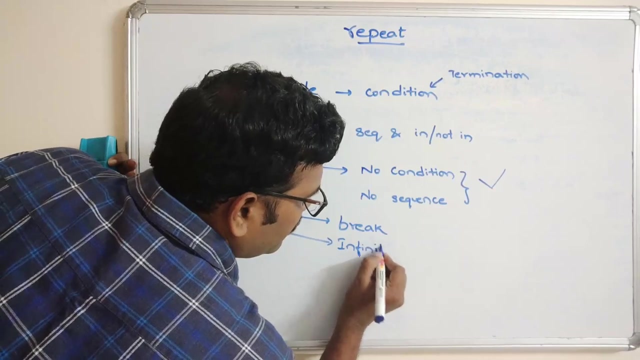 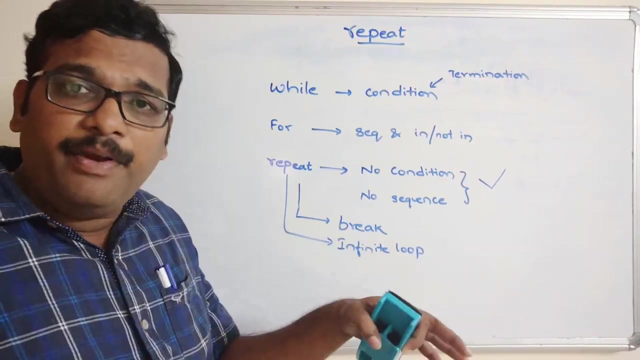 the instructions will be terminated if we use this repeat. so the instructions will be terminated with a break statement. with a break statement, that means this repeat is always infinite loop, Infinite loop. this repeat is always an infinite to, and the infinite loop will be terminated only with the help of a break statement. so the same way. the 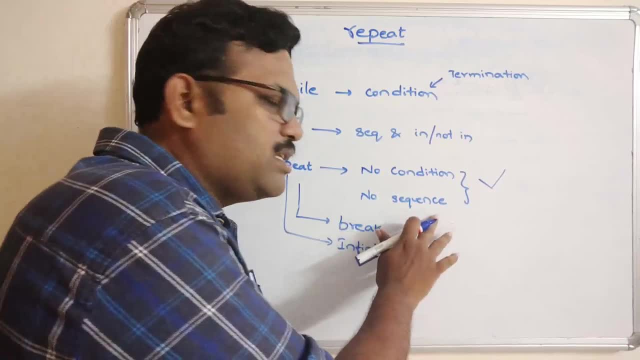 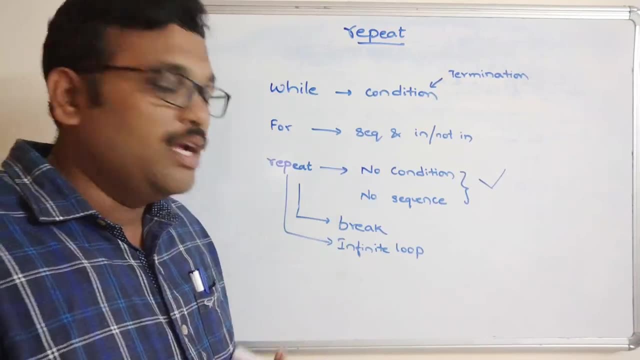 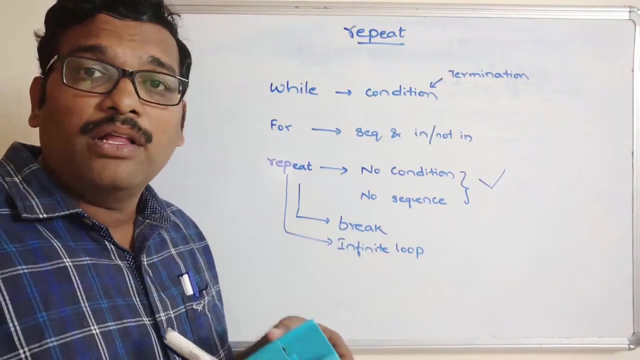 repeat, we are not writing any condition, we are not writing any sequence and just by using the repeat keyword we are going to execute the same set of instructions, multipliers times, so whenever, until until the break statement is getting executed. so we have already seen the importance, the syntax and the working of break in of in our 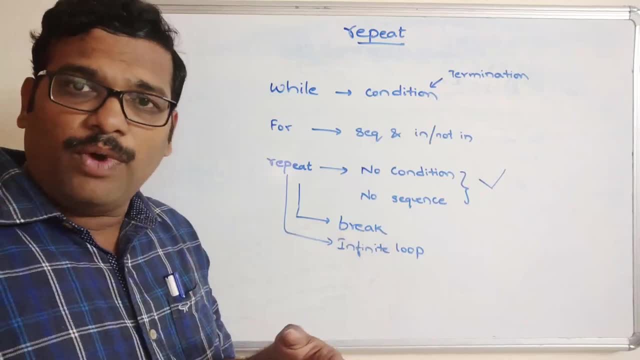 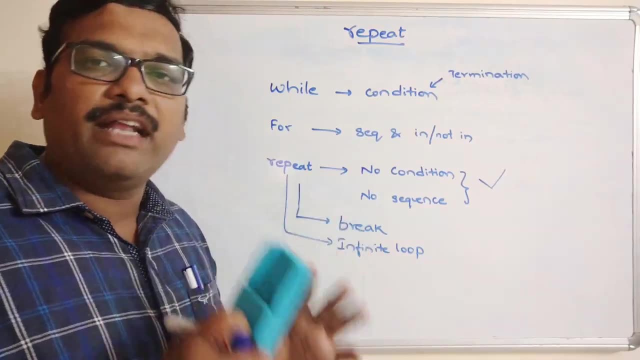 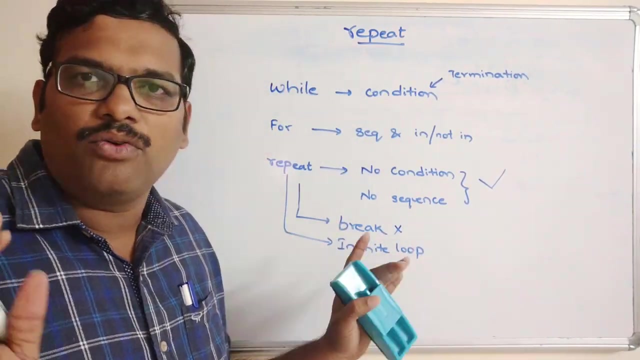 previous session, right. so once go through that one and see, whenever the controller executes this break, immediately the loop will be get terminated. so in the absence of this break, in the absence of this break, the repeat will be always an infinite row. okay, so here the syntax is the syntax. 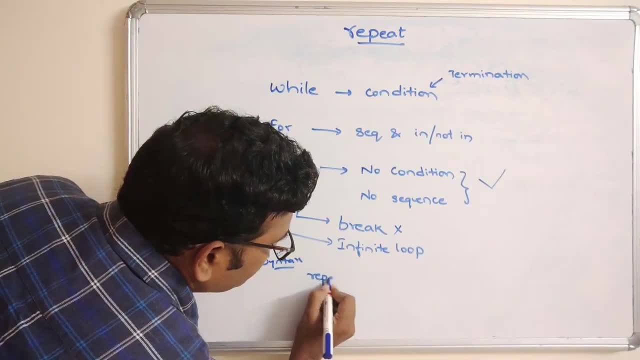 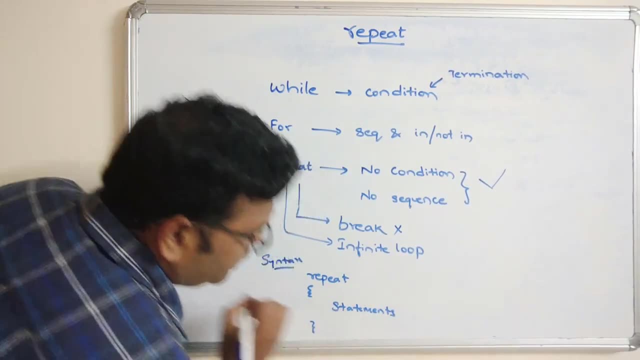 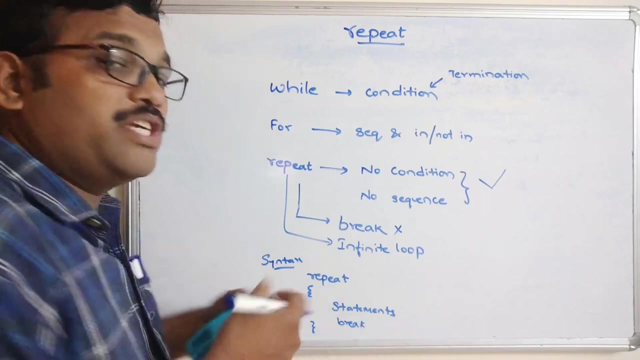 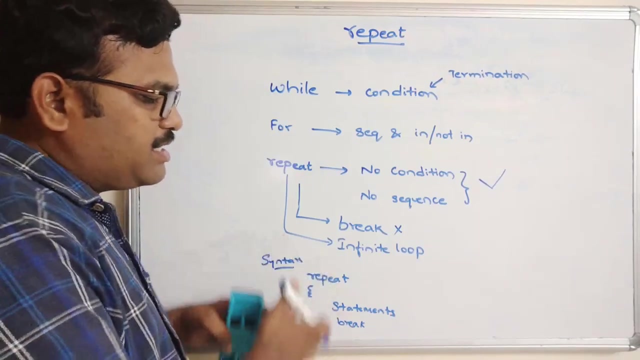 for a repeat is: repeat and do the statements. here repeat and do the statements right. and here we need to write some break. we need to do some break, so we need to check for some condition and we have to include that break. so whenever the condition becomes true, then this break will be get executed and the instructions will 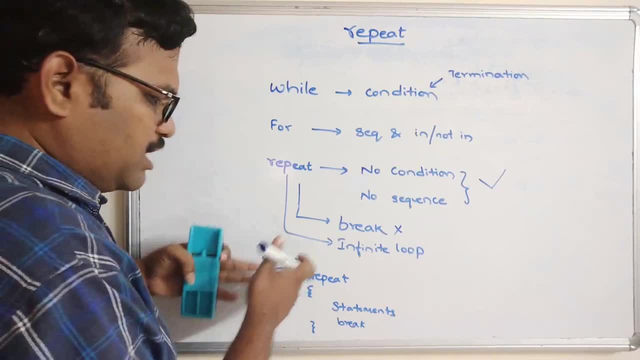 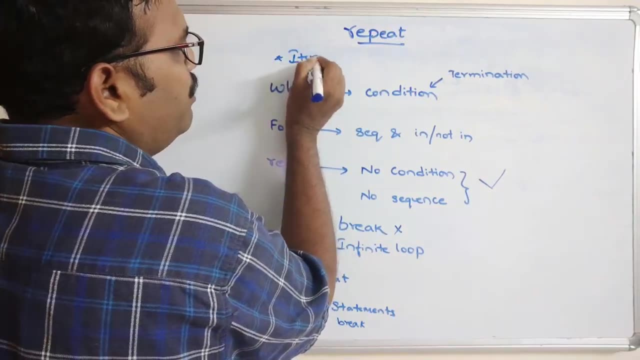 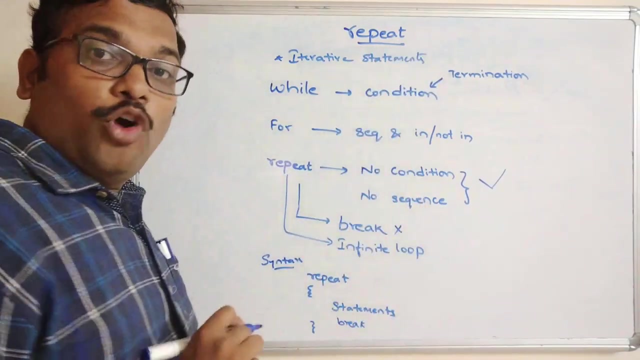 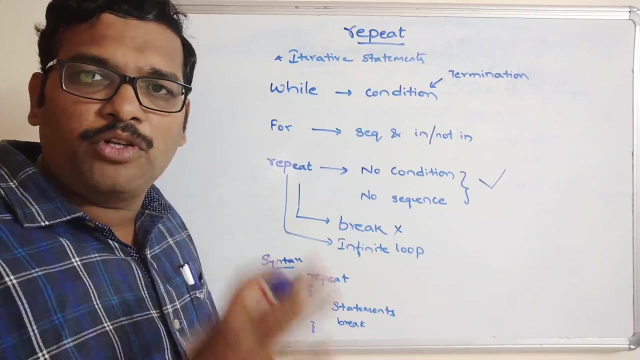 be. the iterations will be terminated, right? so this is a simple syntax for repeat. so this will also be a category of iterative statements- iterative statements- right? so hope you understood the syntax and the working of repeat. now we'll move on to the system and I will demonstrate the working of repeat in. 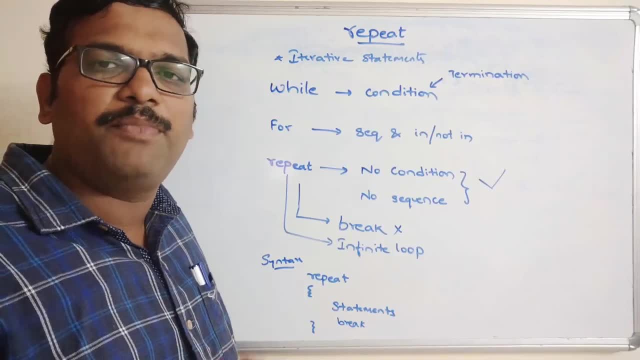 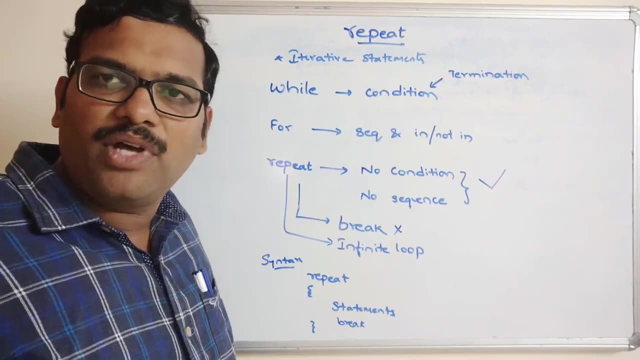 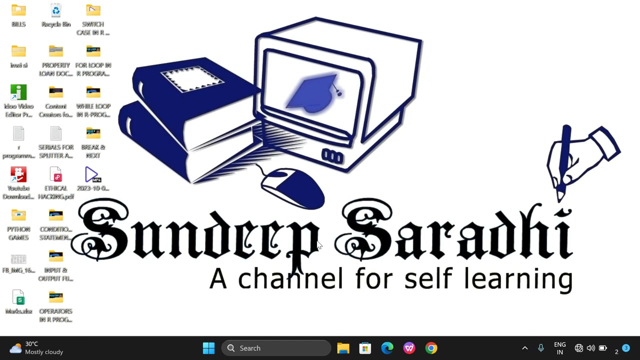 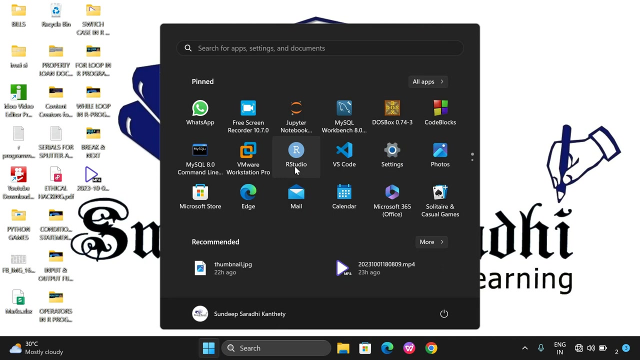 by executing a small program. taking a small example, and execute so that you will be understanding the working of repeat statement. let's move on to the R studio. hello friends. so just now we have seen the syntax of a repeat statement. now we'll see a small example and I will demonstrate the working of a repeat 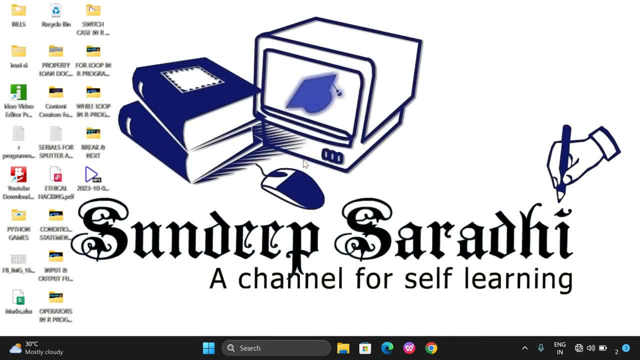 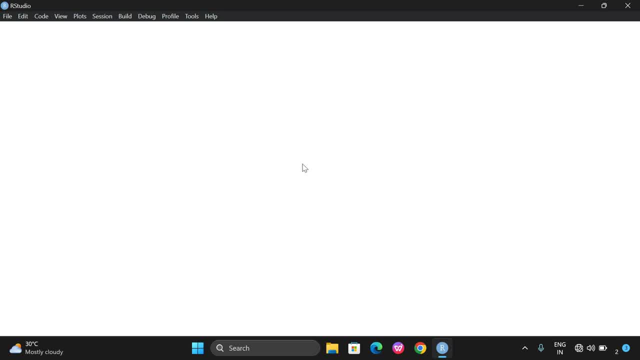 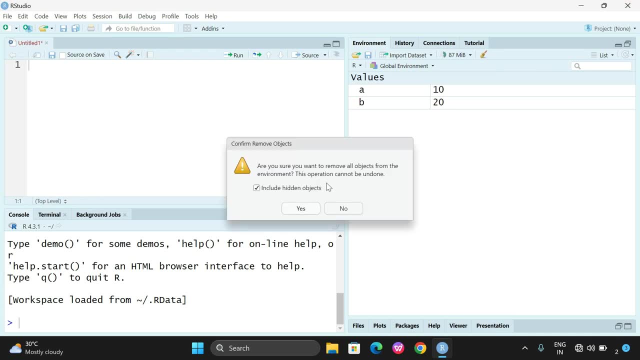 statement in our programming. so let us start with the R studio. so let me open that and let me erase the previous content which is available, both the inputs and the program, and then we take the example, small, small example, so I am clearing all the previous contents. yes, now let us take one loop variable. I'll take loop. 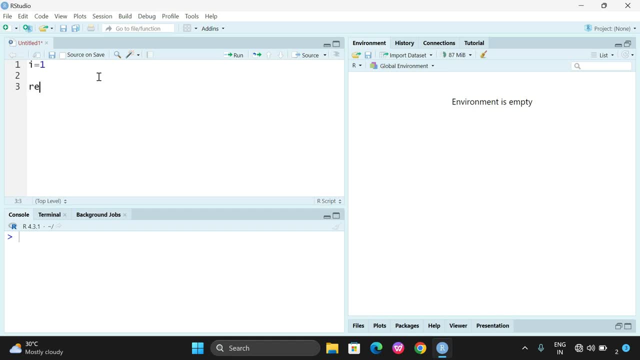 variable, as I is equal to 1 and I will repeat, I use a repeat and here we need to print I and I'll go with the I plus 1, so what happens here? so this is the instructions we are giving. these two are the instructions we are giving inside the 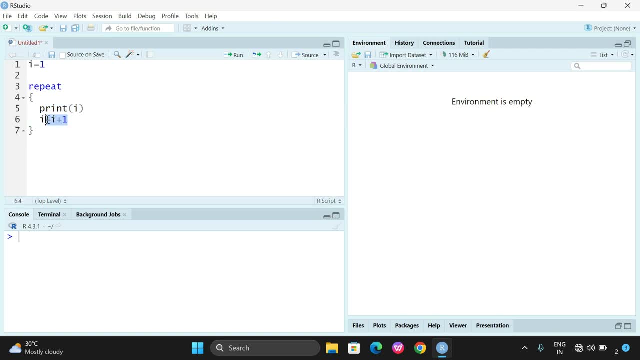 repeat statement, so that means these two instructions will be repeatedly executed, right? so here, not, we are not writing any condition, we are not writing any sequence, So this will lead to infinite loop, For example. see, this will lead to infinite loop, So it will start with 1. and see, you can observe, just moving on with a lot of numbers, right, This? 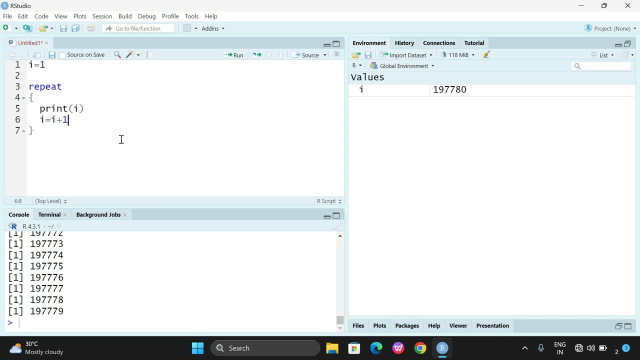 is an infinite loop Now. so, without any condition, it will be an infinite loop. So you can see, I will write here. I will write if i is equal to 10, let us take it as a break. Okay, now you can execute here you can see 1,, 2,, 3,, 4,, 5,, 6,, 7,, 8,, 9,, 10.. So